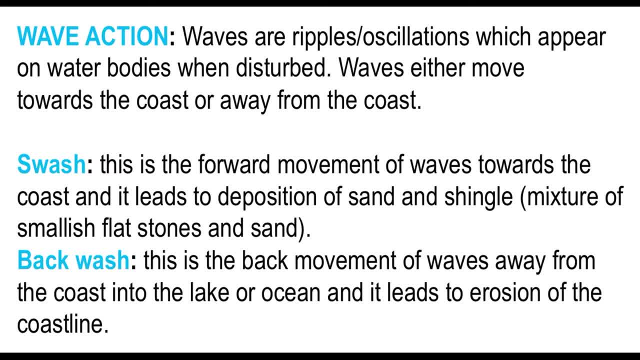 sand shingle, which is a mixture of smeltshe flat stones and sand, Then the backwash. This is the back movement of waves away from the coast into the lake or ocean or sea and it leads to erosion of the coastline. 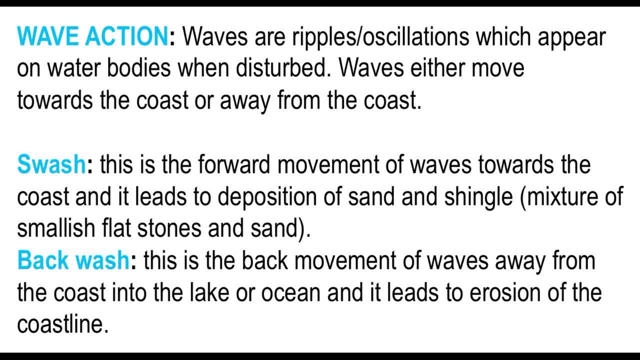 So the swash that we have talked about is where now, water as waves move from the water body to the coastline, and then the backwash is where these waves move back away from the coastline and they do form different futures. the waves that we are seeing now, the one that goes towards the cost that 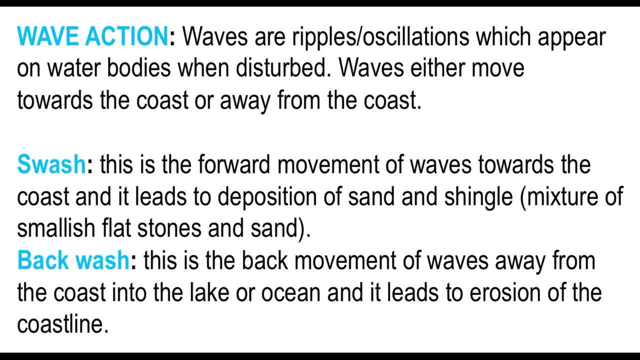 deposits and the one that goes off the cost that erodes cause different futures. so in this processes right now we are saying we have to the swash that we are seeing here that move towards causes what we call depositional wave futures. then the backwash causes all forms what we call wave erosion futures. in this 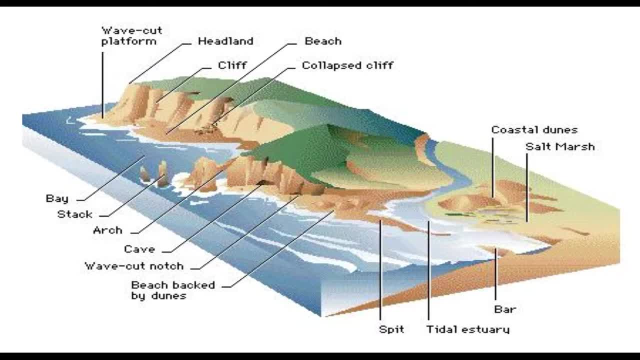 illustration. right now we can see a simple illustration of a coastline accost and the futures- I write it here- are the ones that we are talking about. in this diagram we have a mix of deposition wave futures and erosion wave futures, highlighting a few. so under the erosion futures we have what we call a cliff. 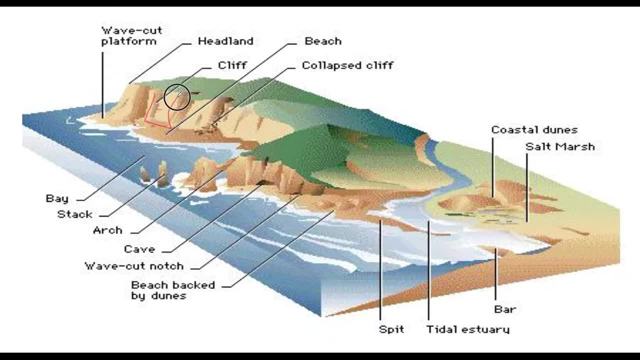 which is this one. this is our cliff. then we have what we call a headland, where land protrudes into the water body. we have what we call a wave cut platform, which is this one here. then we have what we call a bay, where water produce into. 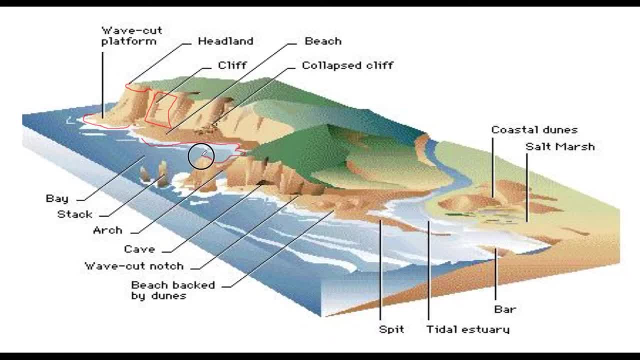 land. this is our bay- coming out. this is the bay where we see water. then we have what we call an arch- these are all futures formed due to wave erosion, where now waves move off the coast. as they do erode the backwash and the waves, we have what we call the constructive and destructive waves. so the arch also. 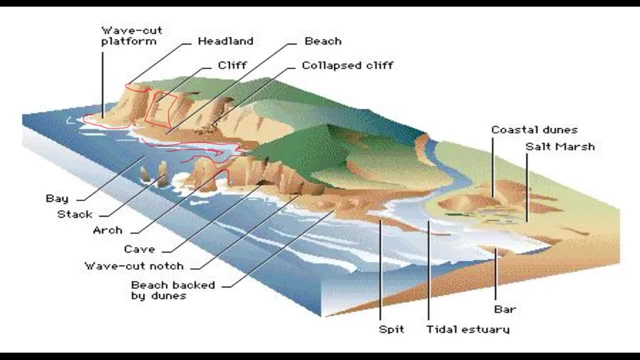 falls into the futures, formed by wave erosion. the stack, too, forms due to wave erosion, and then all these are also, which means wave and Gravity, such as clay and water, all these faces that we see here performing due to their motion, much so. adding on is the ны, Nebraska. 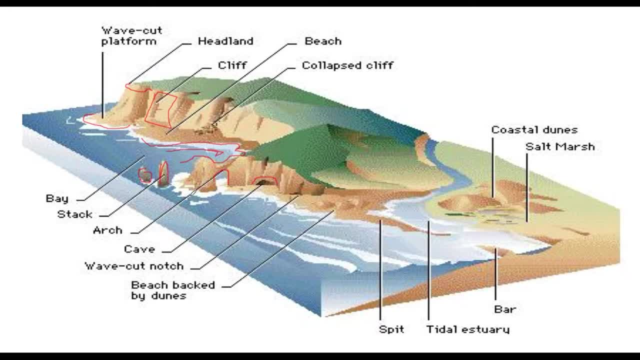 and beasts of formed due to wave erosion. so will we see this with the Roe de esta Olis, м meters of 350 km away, as it turns by J Eigen? the process of attrition, hydraulic action. it's fairly developed, but in the middle and to maybe one of the three不是. 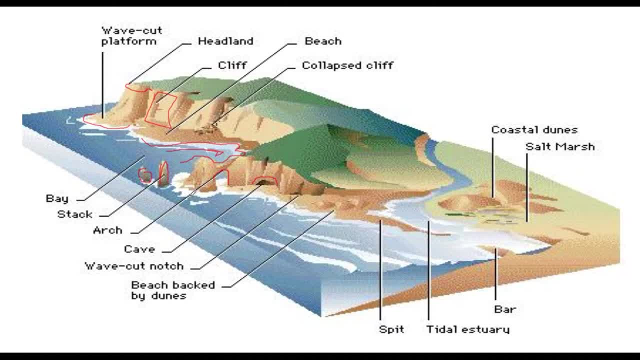 abrasion and solution. those processes lead to what we call erosion. then we are talking about deposition. in the same illustration, right here, we are also having features formed by wave deposition. for example, the beach. this is our beach, and the beach is what we see here, where we see this sand, those who 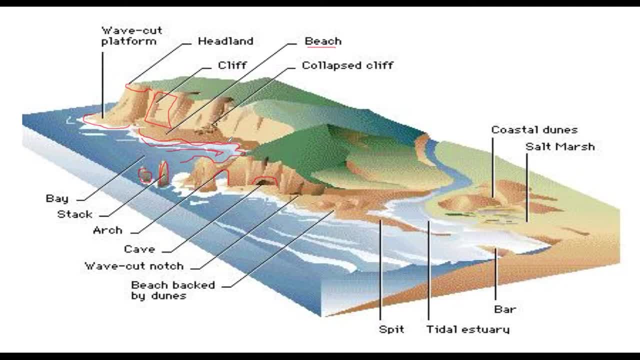 have ever gone to the beach to relax, we have what we call the dunes, the sand dunes around this area deposited. as we said, waves deposit different materials, for example the sand, the gravel and the boulders, plus silt, as we shall see. So here, waves are depositing what we call sand forming. 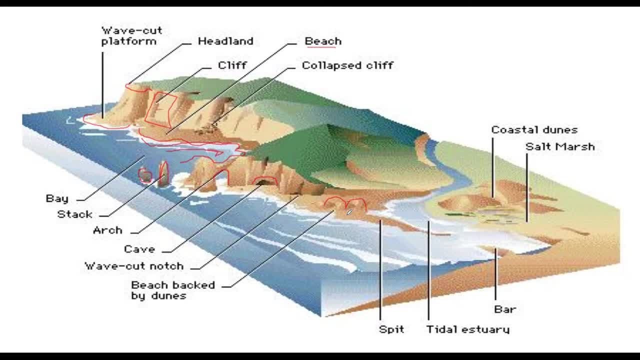 the sand dunes. We also have what we call the salt marsh, this area here, which is here. These are salt marshes. We also have what we call the spit, where we see the sand protruding into water due to the oscillation of these waves, And this is our spit. This is the spit. 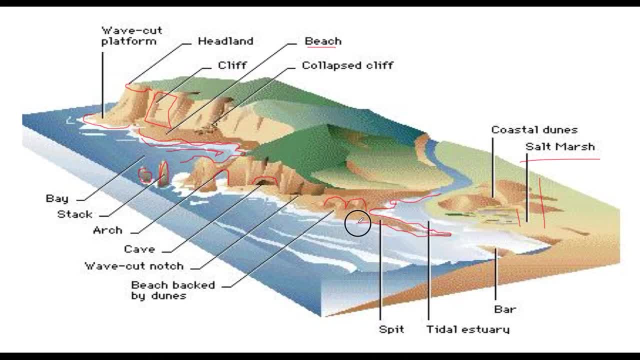 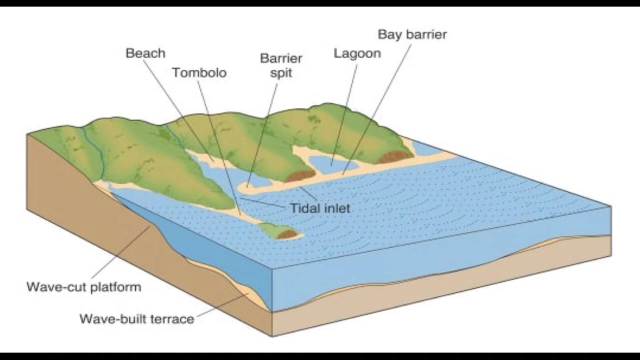 that we are talking about, where we see sand. this is our sand protruding into the sea or the lake. So this is spit and these are features formed due to a deposition. To add on more to those features, we have what we call the tombolo, which is here around. 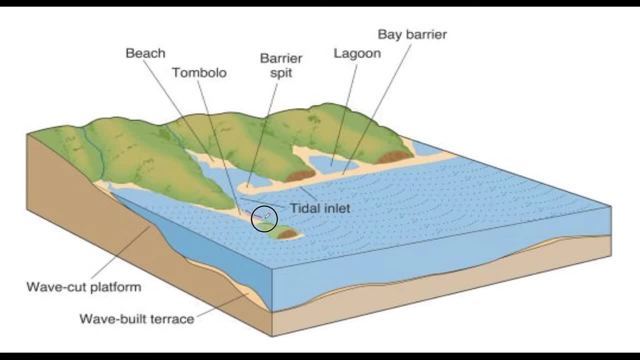 that area- This is our tombolo- where we have sand and quite some vegetation. around this area We have what we call a lagoon, where a calm water is formed off the main water body into the land due to deposition of sand. 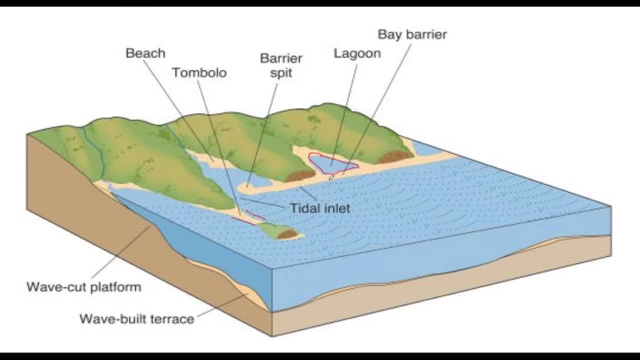 And this is our barrier that separates off that calm water from the main water body, which is this one: This is our main water body and then this is our lagoon calm water around that area. So we have what we call also the barrier spit. 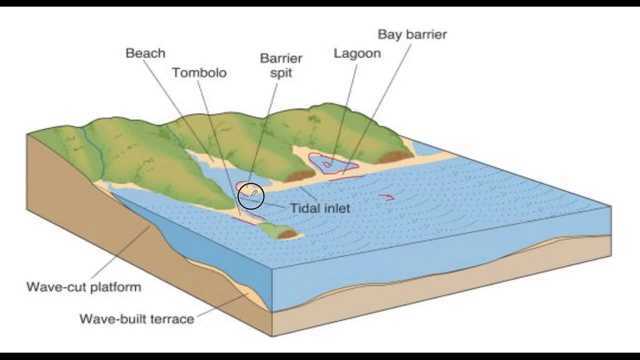 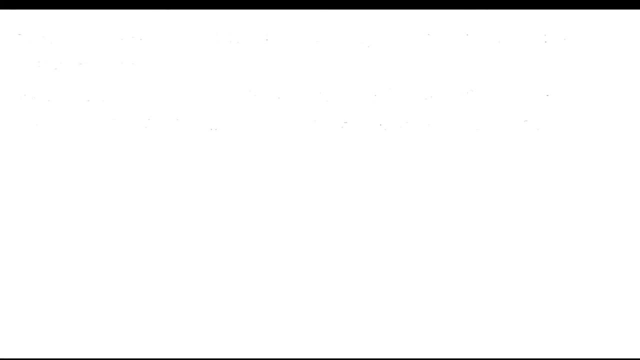 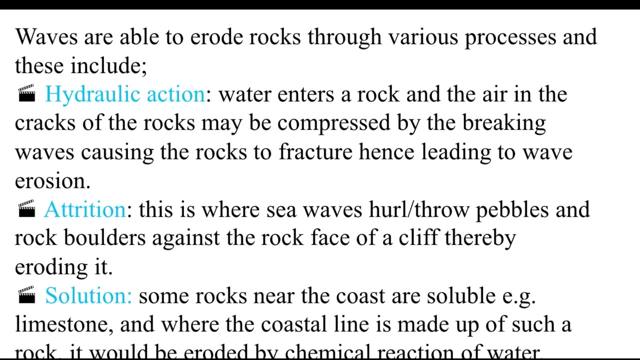 This is what we have just talked about in the earlier illustration. This is our spit, where we see sand being deposited around this area: Wave action. Waves are able to erode rocks through various processes, For example hydraulic action, where water enters rocks cracks and air in the cracks may be compressed by. 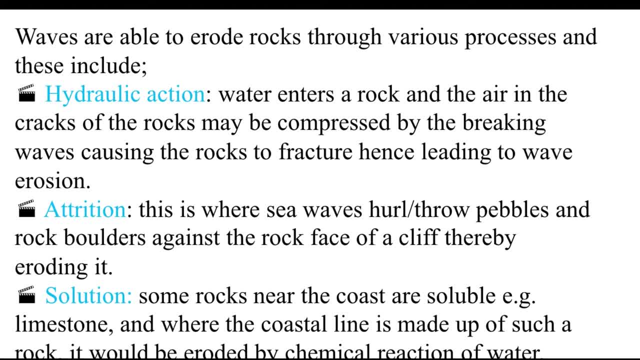 the breaking waves causing the rocks to fracture The attrition. This is where sea waves hollow or throw pebbles and then rocks. borders again are the rock face of a cliff, thereby eroding it. This is where intense and strong waves throw the hard rocks onto the face of the cliff, banging it, and 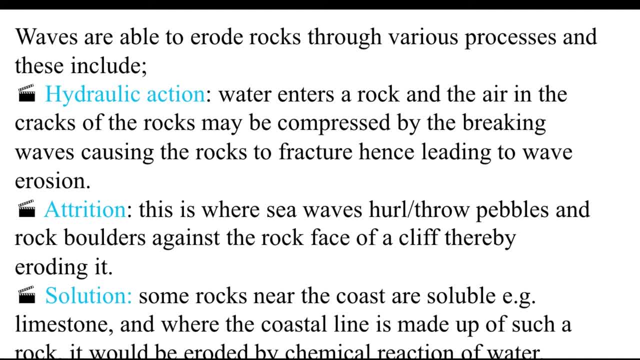 hence cracking it slow but sure, causing what we call erosion. Lastly, we have what we call solution. Some rocks near the rock coast are soluble, for example limestone, and where the coastline is made up of such a rock, it would be eroded by chemical reaction of the water It forms and then it melts, dissolves into water. 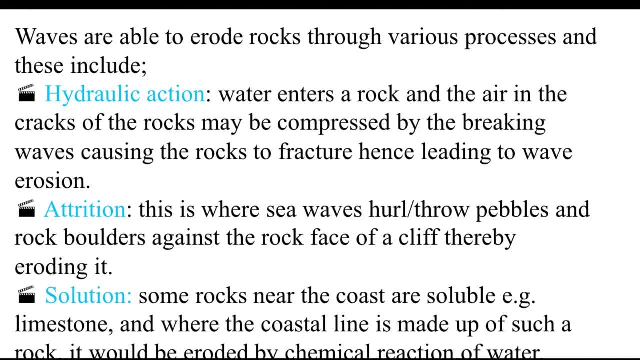 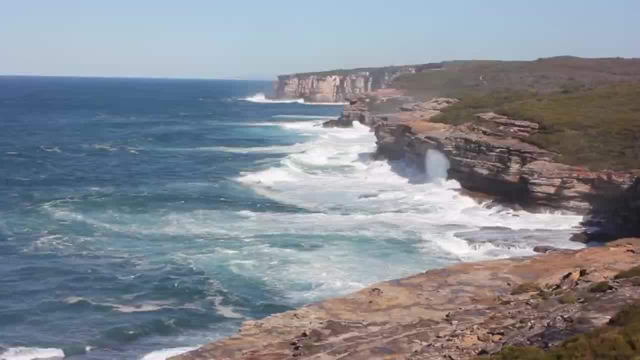 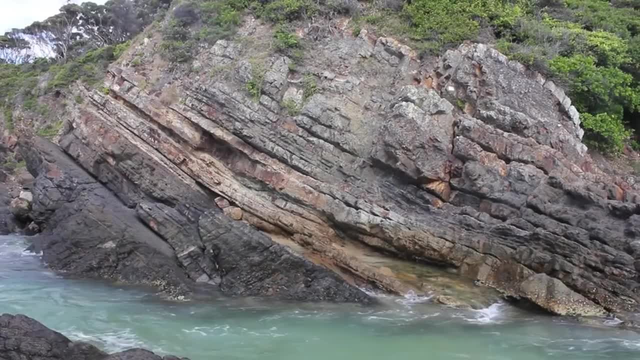 forming a solution and is easily eroded, For example, the limestone rocks. Features formed here include the arch, the cliff, the wave cut, platform bays, headlands, caves, arches, stacks and stumps. So we're saying: a cliff is a steep slope of a 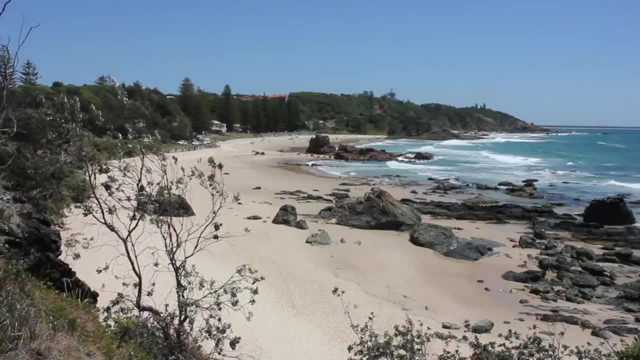 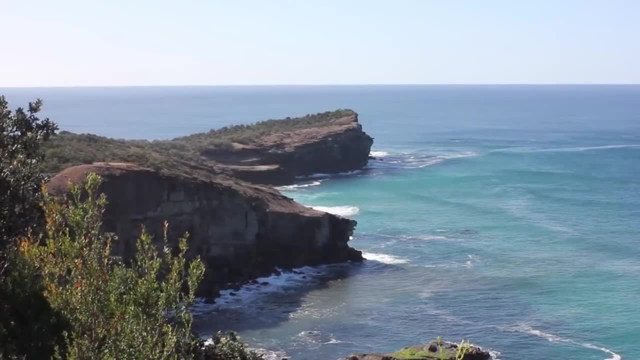 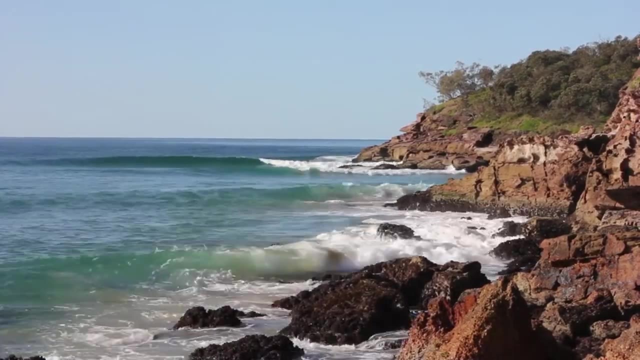 rock face along the sea coast. It is formed as a result of waves eroding highland along the coast through a process like hydraulic action, where a cliff tends to be undercut and, in the time of the upper part, collapses into the sea under its own weight. 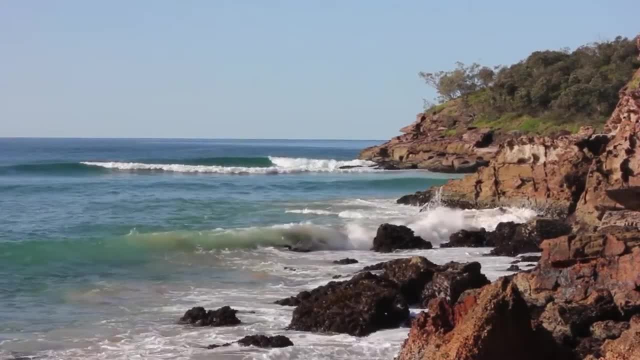 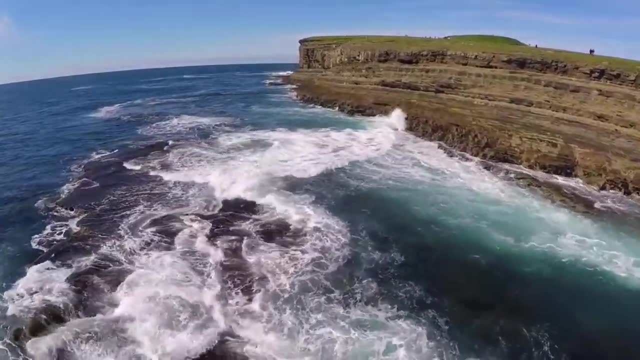 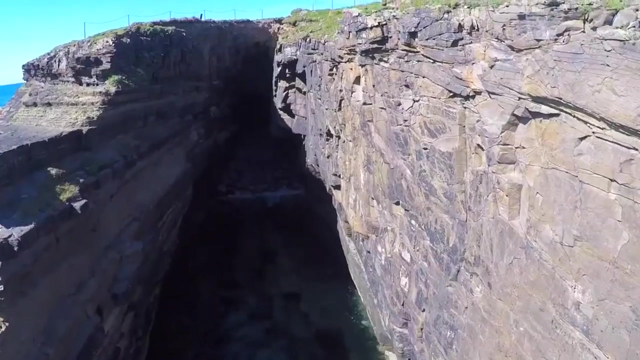 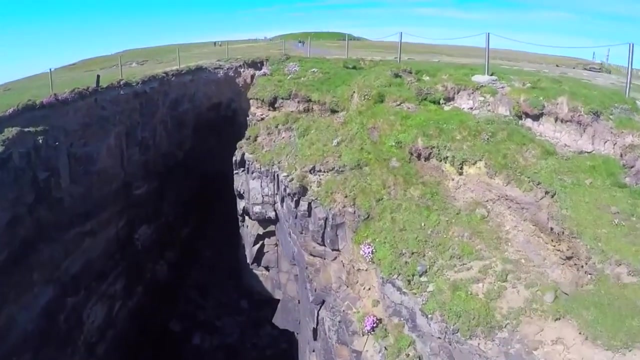 Wave cut platform. these are formed as a result of attrition. where we see a cliff, recession takes place. The base of the cliff is left behind as a platform over. the rock Materials deposited from the cliff may be deposited on top of this terrace like forming features. and we're saying wave cut platforms are often visible only at low tide or 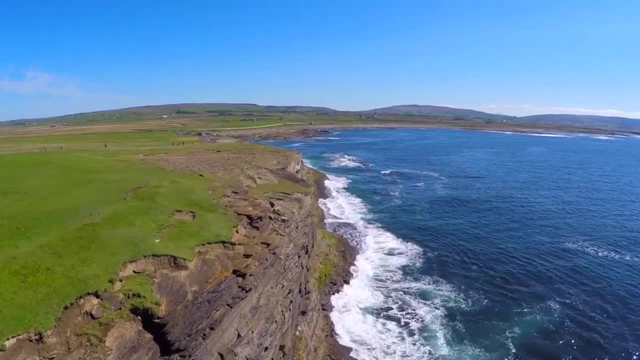 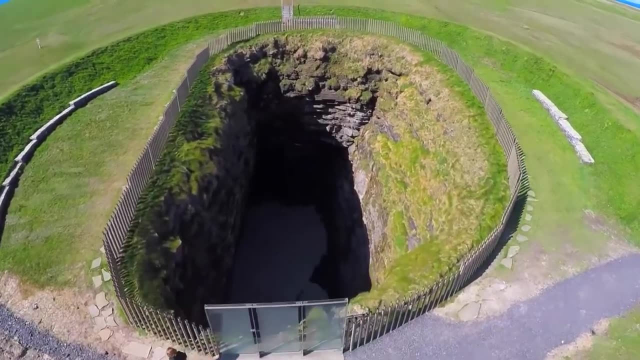 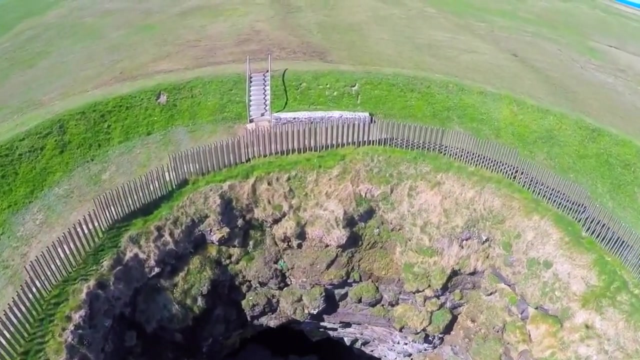 high tide Bays and headlands. these are formed in areas along the coast where a soft rock lies between the areas of hard and soft rock. The sea does not erode soft rocks evenly with the hard rocks. Definitely, the softer rocks are easily eroded compared to the hard rocks. And what 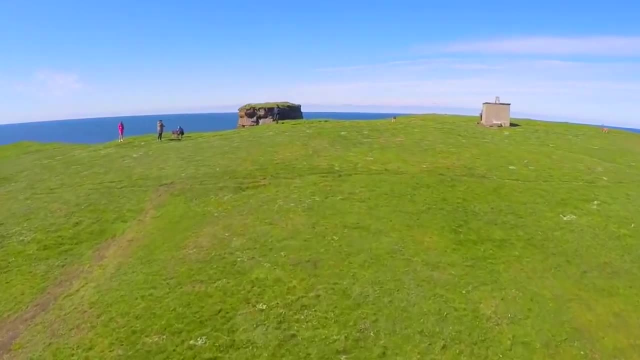 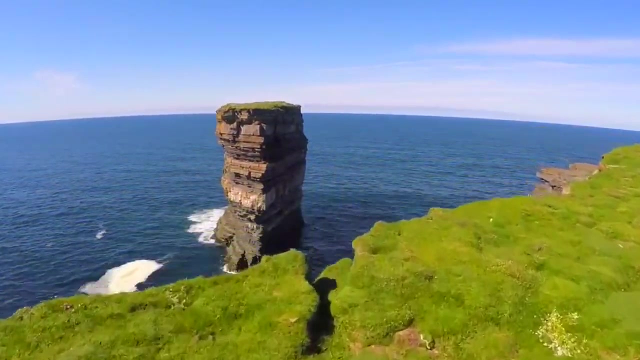 we can see here is the sea has acted on this land and has formed different features. For example, the sea has formed a rock that is connected to the other rock. The sea has formed a rock that is connected to the other rock. The sea has formed a rock that is connected to the other rock. 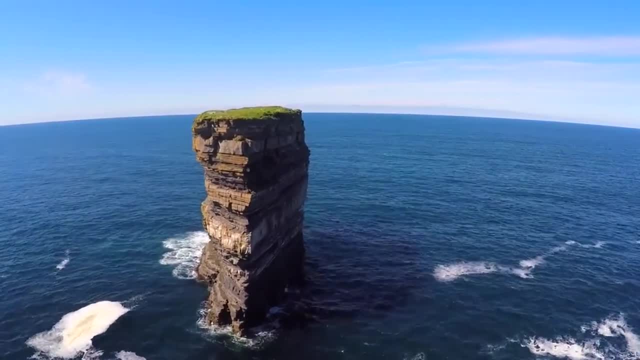 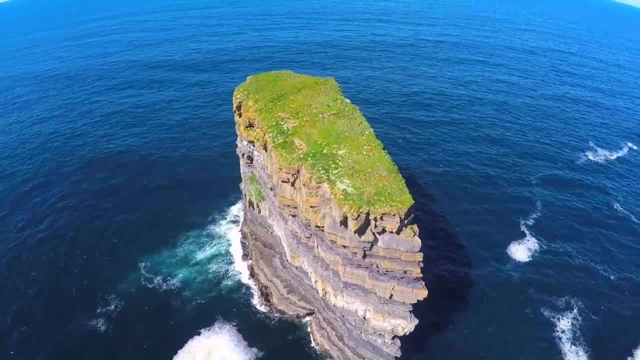 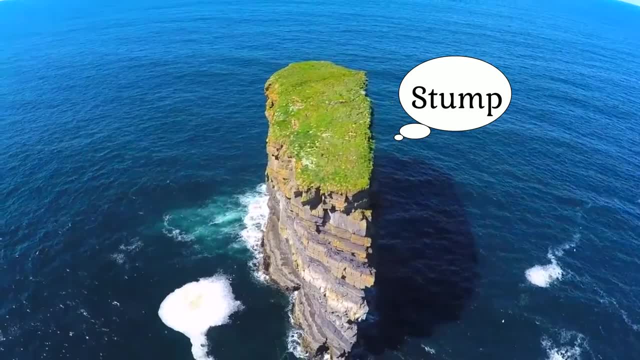 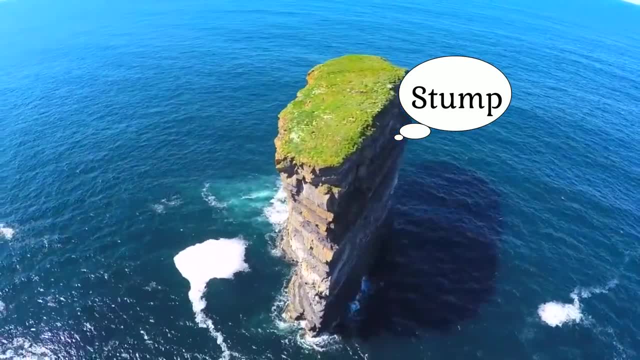 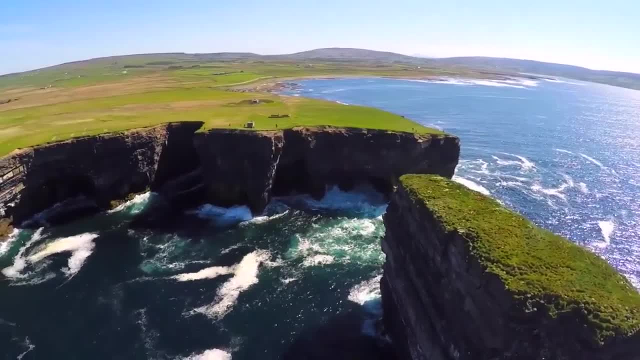 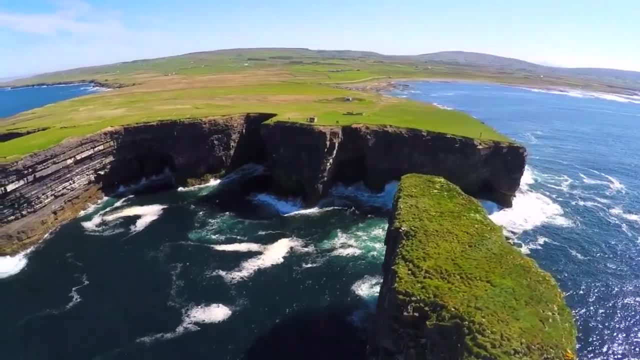 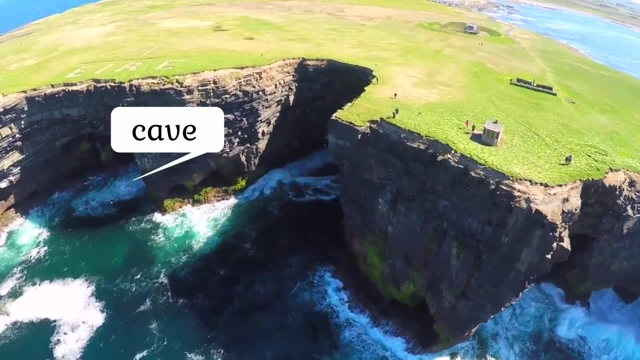 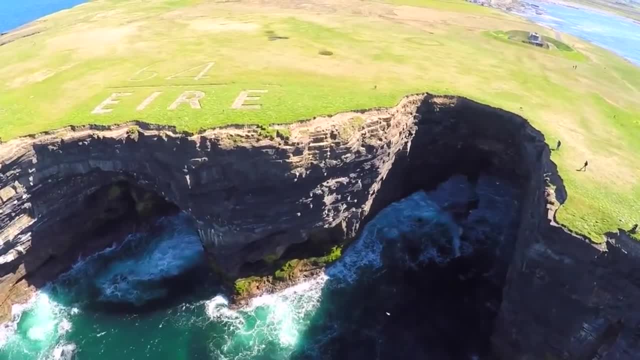 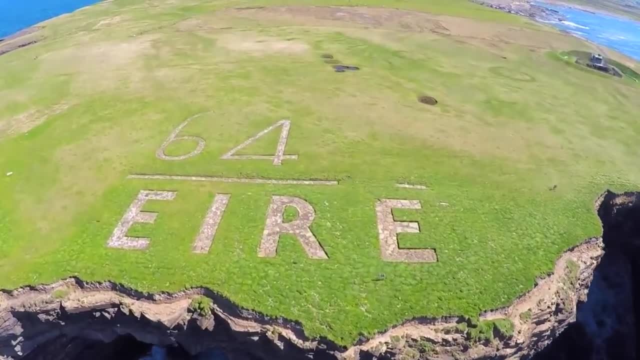 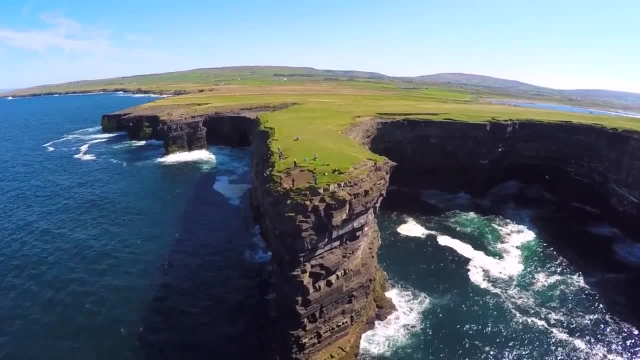 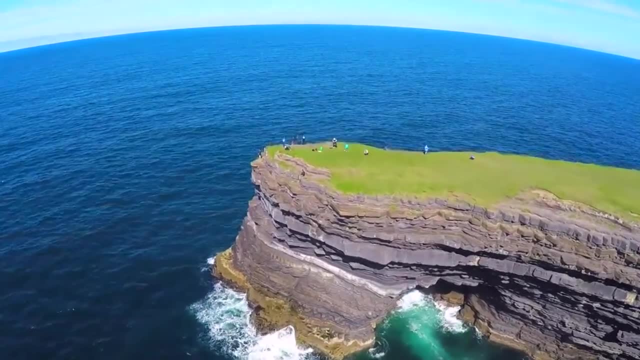 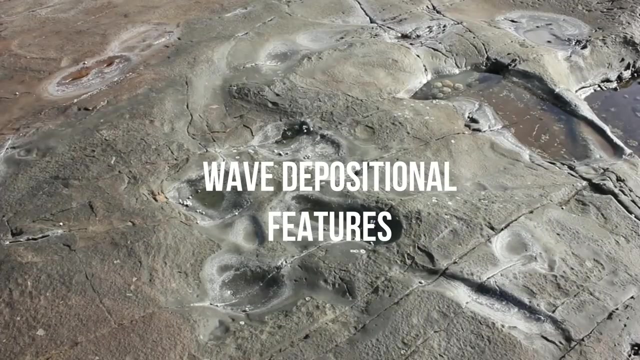 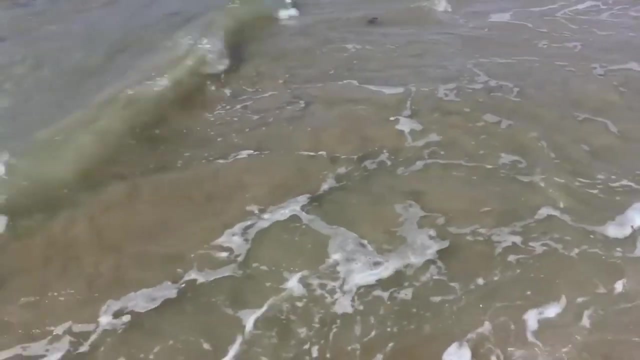 the mainland or the coastline continuously eroding it, forming different futures that we have talked about. What we see right there is wave erosion taking place. This mainland is soon reducing in size. Let's move on to wave deposition of futures. These are futures formed where we see waves depositing different materials on the coastline. 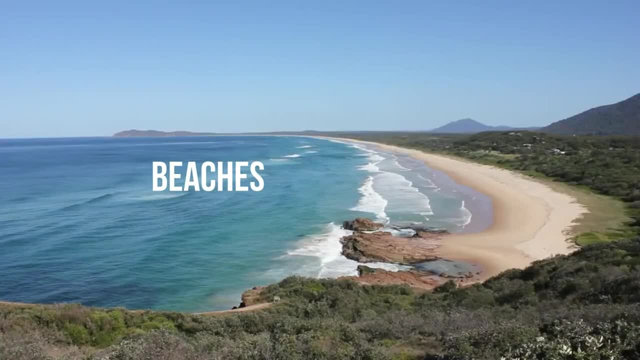 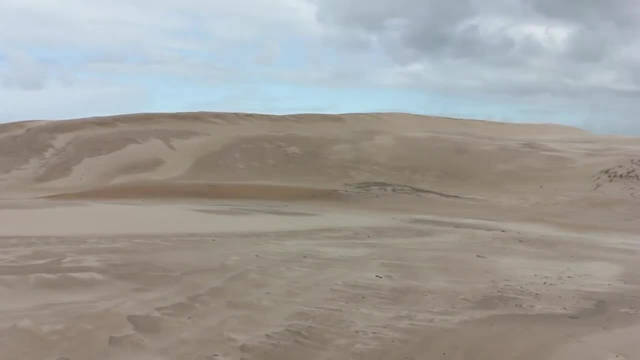 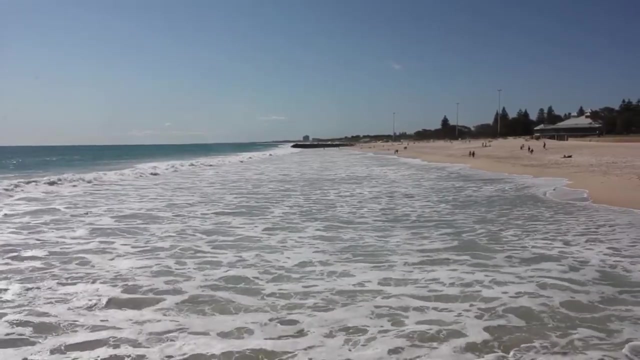 So we say the backwash erodes the swash dust deposits, For example, the beaches that are formed, as we can see down here. This is the main area formed due to the deposition of the sand, The sand dunes that we have just seen, the tombolo that we are seeing right here. 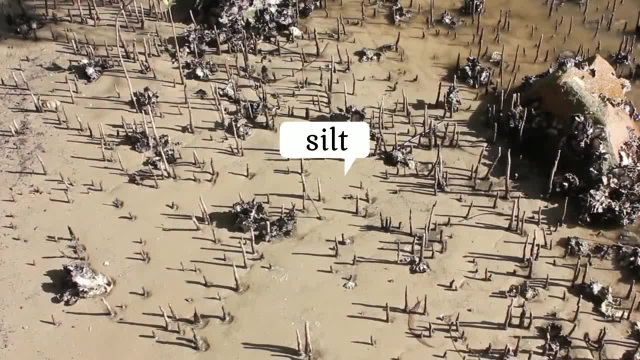 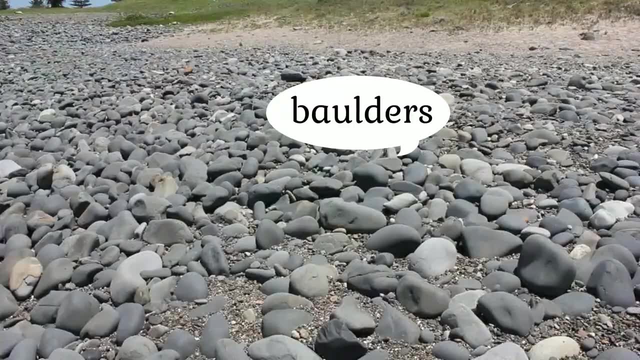 These are futures formed due to wave deposition. So what we see here is silt deposited by the waves, And then we see sand, And then we see gravel, And then we see boulders. These are the features formed due to wave deposition. 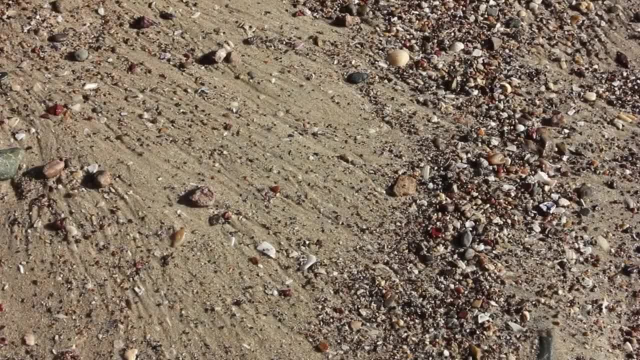 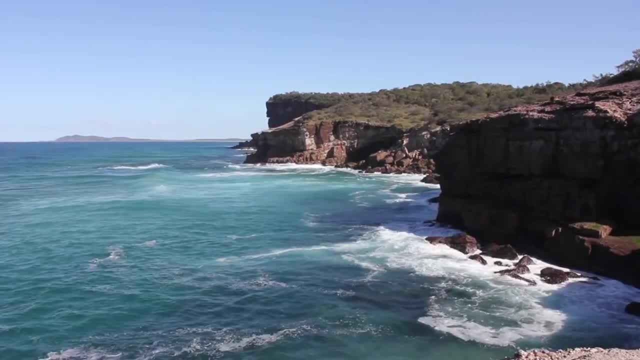 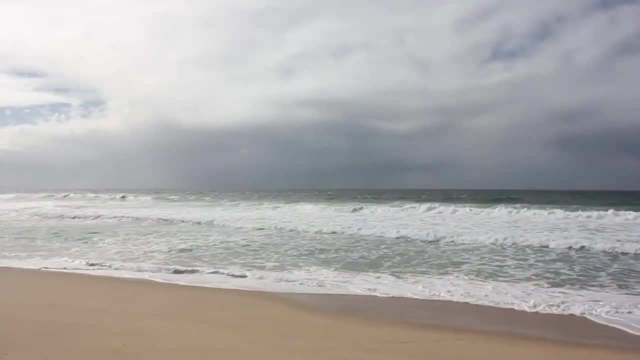 Different materials are deposited due to different types of rocks around the coast, as we can see there. So we have softer, harder, quasite limestone, different rocks. So the deposition depends on the different types of rocks, As we said that the waves are different types.